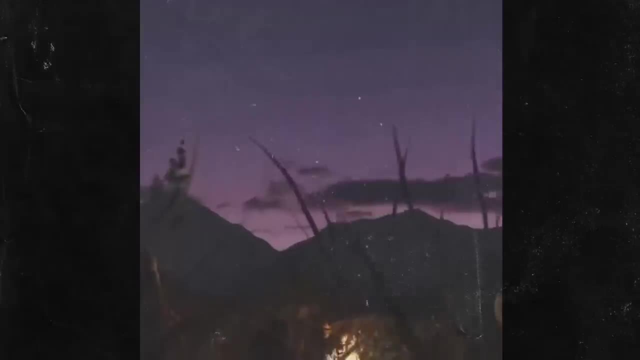 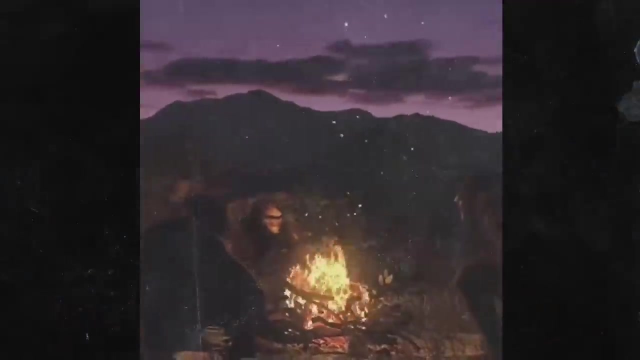 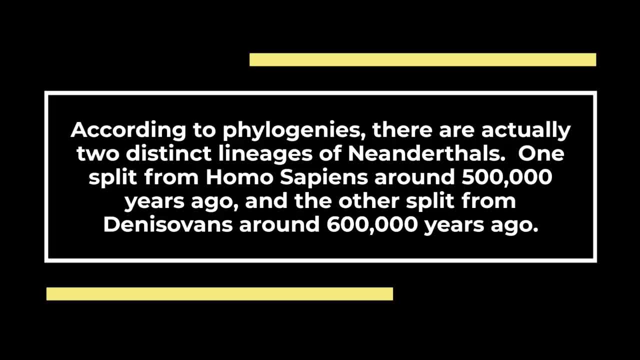 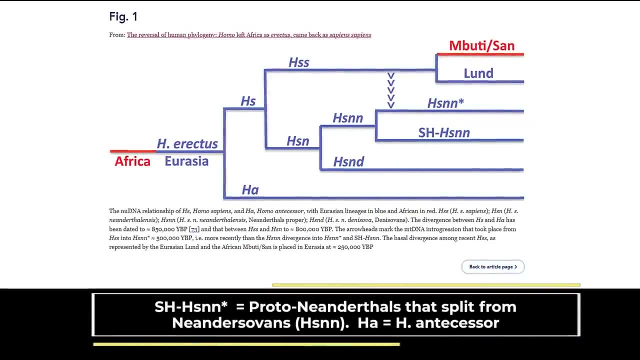 According to phylogenies, there are actually two distinct lineages of Neanderthals. One split from Homo sapiens around 500,000 years ago and the other split from Denisovans around 600,000 years ago. This lineage that split from Denisovans, called the Proto-Neanderthals, is known only from 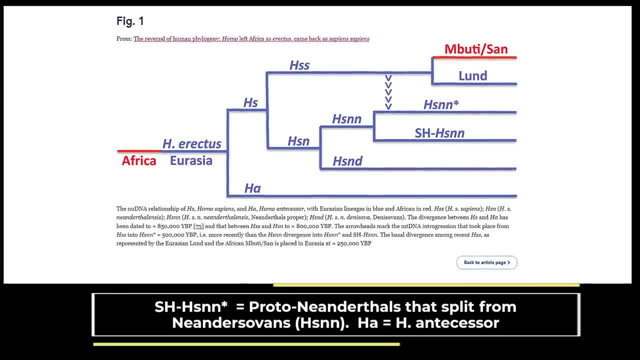 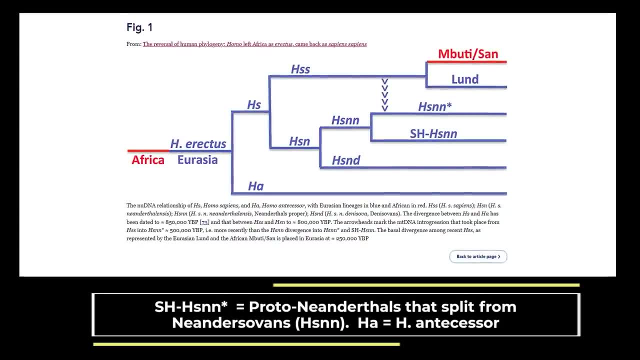 fossils found in Spain and died out or was absorbed into the later Neanderthals group. This begs the question: did the last common ancestor originate in Spain? Most likely this common ancestor was an offshoot of Homo erectus, which, in one of 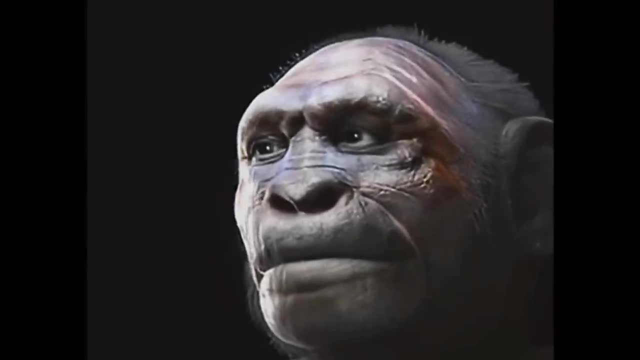 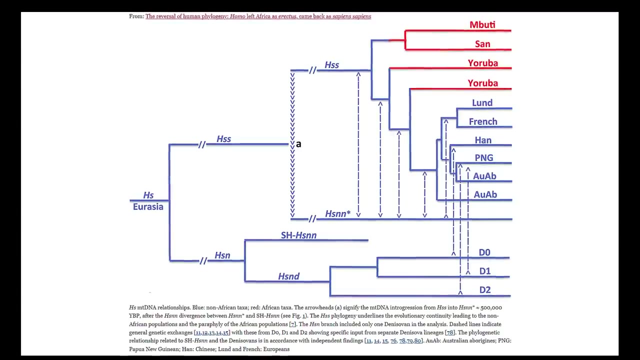 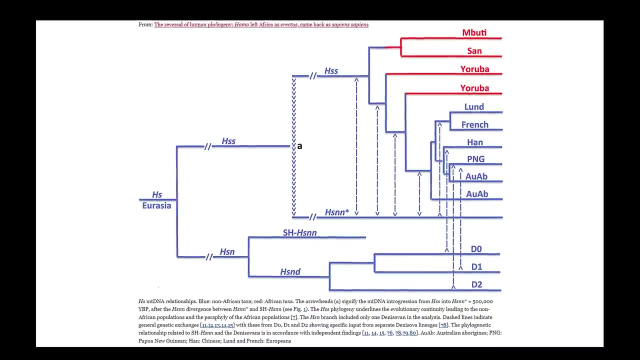 my previous videos, you learned is known as Homo sapiens erectus. This phylogenic tree shows the relationship between these groups, which split up around 850,000 years ago. The Oceima de los Juzos, hominin of Spain, previously thought to belong to another ancient. 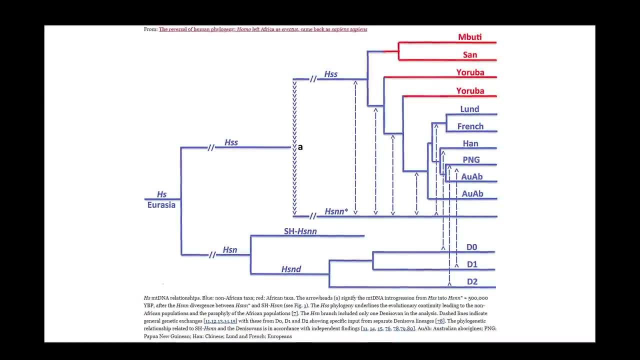 human species known as Homo heidelbergensis. Now scientists say that the hominid family of Homo heidelbergensis is known as the Homo de los Juzos hominin, which was found at the Spanish site of Oceima de los Juzos is. 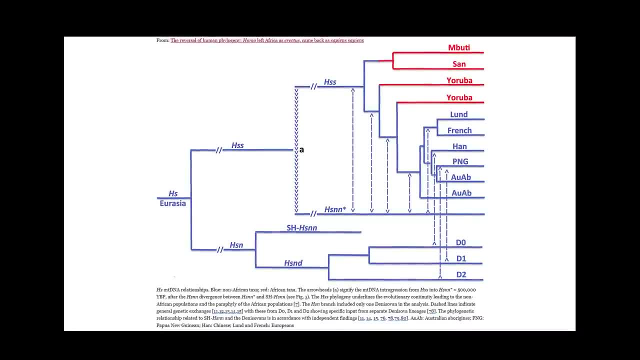 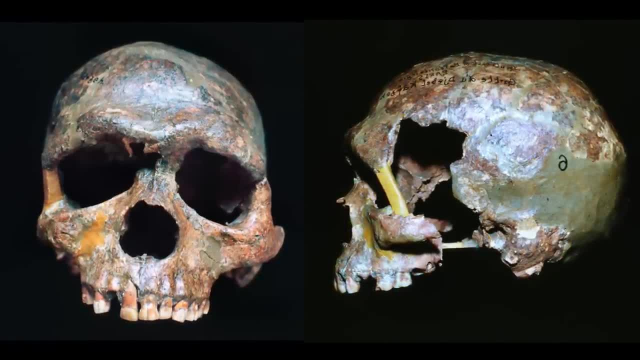 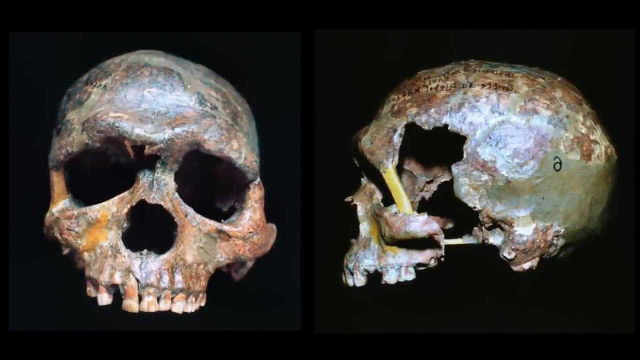 a Proto-Neanderthal. Indeed, an interesting question is how these Middle Stone Age hominins were related to those who lived in the Late Stone Age epoch, in particular to Neanderthals in Western Eurasia and to Denisovans, a sister group of Neanderthals so far known only from a DNA found in a finger. 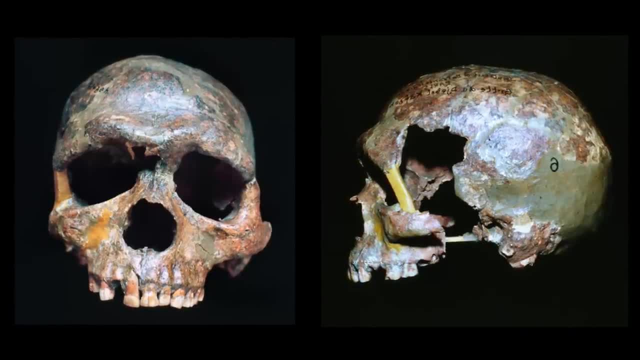 bone, a mandible and a tooth found recently in Laos. Previous analyses of the Oceima de los Juzos hominin showed that their metastases were found in the late Stone Age epoch, in particular to Neanderthals in Western Eurasia and to 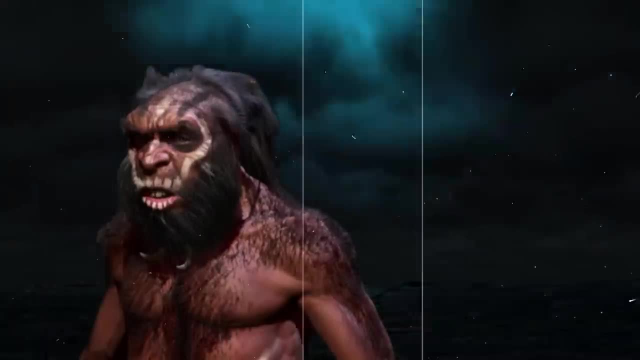 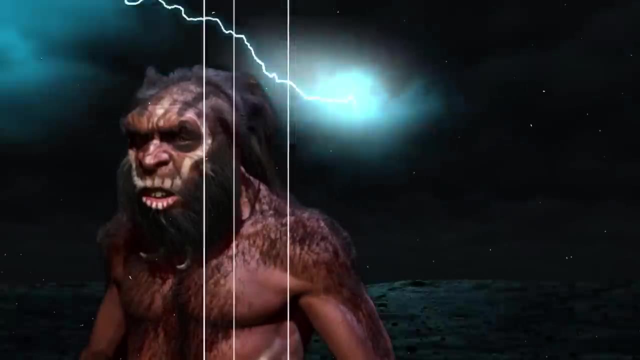 Denisovans in Western Eurasia. The results of these studies show that their maternally inherited mitochondrial DNA was distantly related to Denisovans, but not closely related to other Neanderthals. The new results show that the hominins were a more ancient lineage of Proto-Neanderthals. 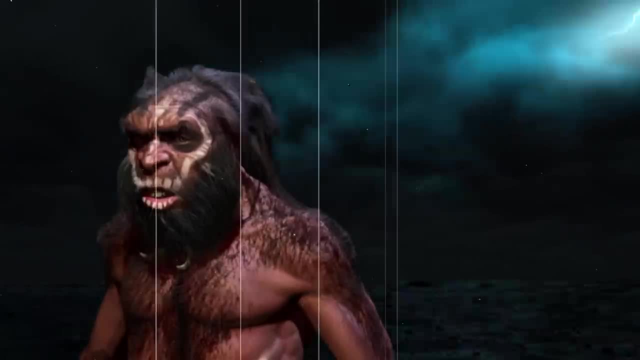 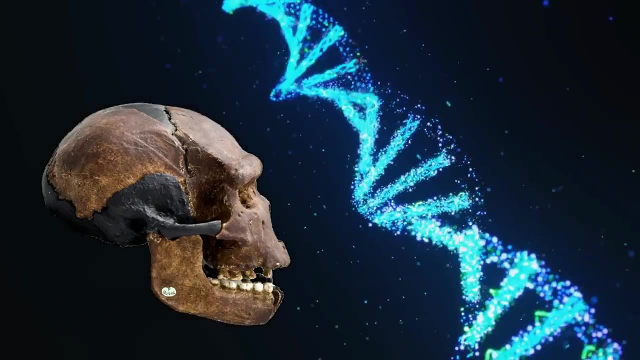 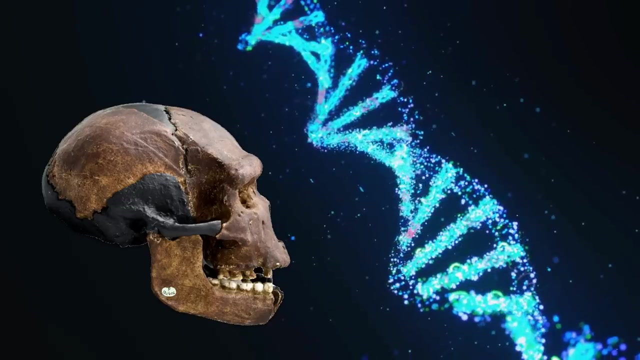 but distantly related to other Neanderthals. Scientists recovered nuclear DNA sequences from two specimens which show that the Spanish Proto-Neanderthals were more closely related to Denisovans than to other Neanderthals. This early Neanderthal-Denisovan lineage, called the Neandersevans, had big brains and 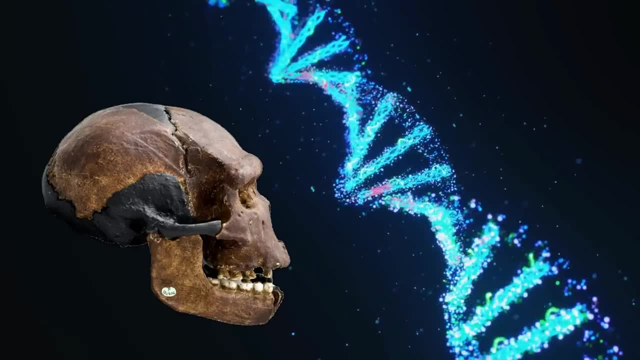 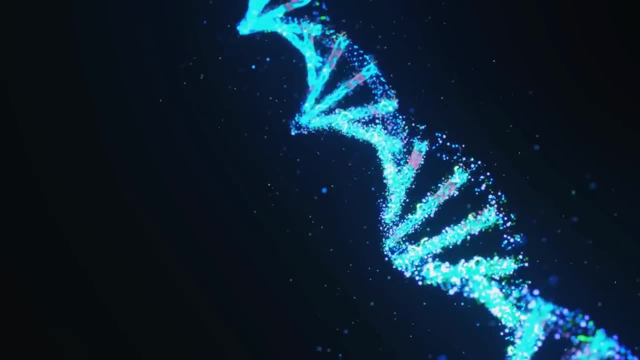 so, of course, did their descendants, the Denisovans. The Neandersevans split about 600,000 years ago into Proto-Neanderthals in Europe and Denisovans in the East. In another study, scientists estimated the date of the Neanderthal-Denisovan split at: 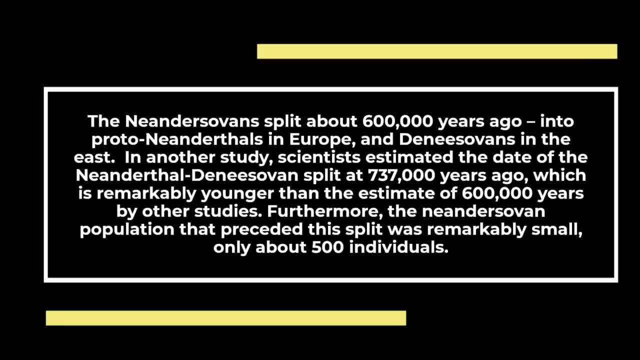 737,000 years ago, which is remarkably younger than the estimate of 600,000 years by other studies. Furthermore, the Neandersevan population that preceded this split was remarkably small, only about 500 individuals. This supports the previous results, which indicated an early separation of Neanderthals. 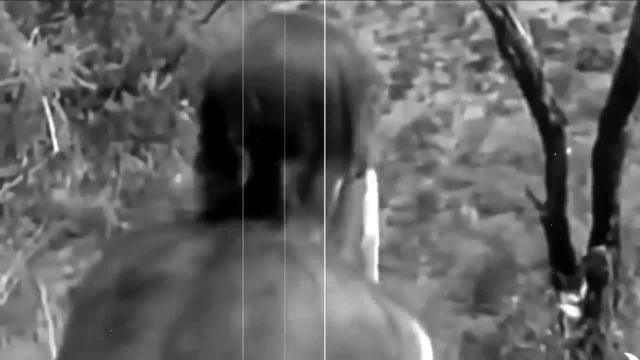 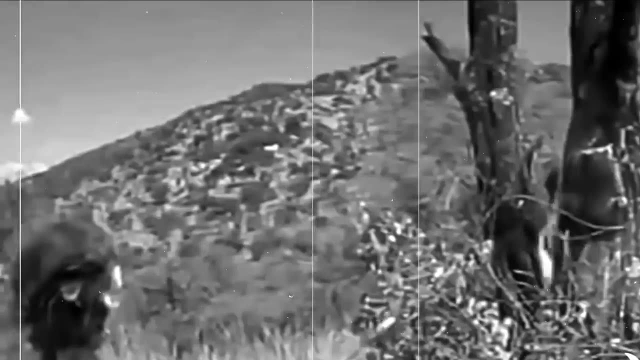 and Denisovans and an Ice Age bottleneck among their ancestors. Nonetheless, these results provide important anchor points in the timeline of human evolution. They are consistent with a rather early divergence of 800,000 years ago of the modern human population. The Neanderthal-Denisovan population was a group of Neanderthal-Denisovan. 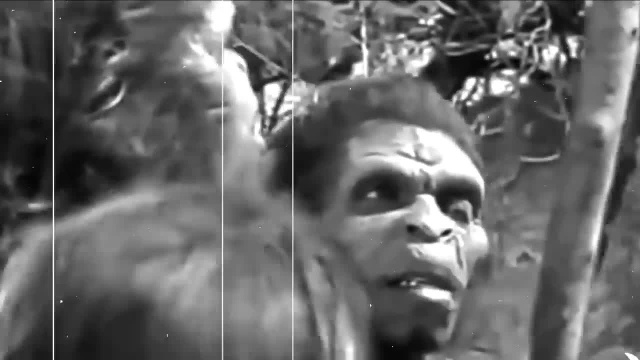 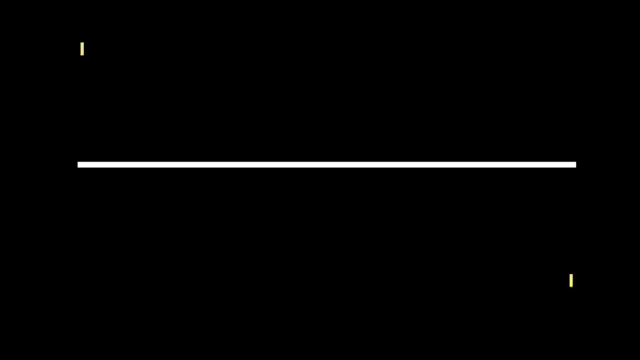 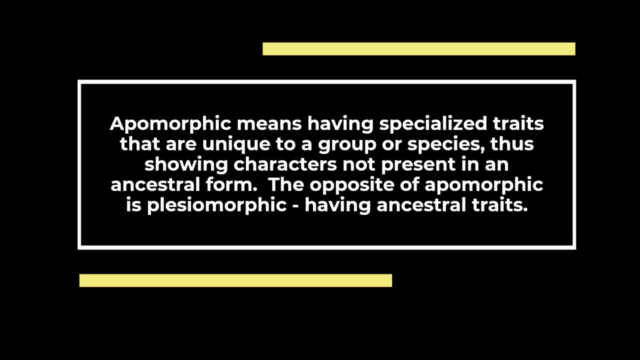 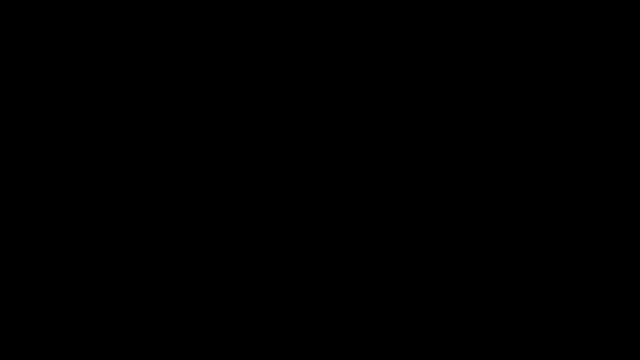 The Neanderthal-Denisovan population was a group of Neanderthal-Denisovan. The Neanderthal-Denisovan population was a group of Neanderthal-Denisovan. TheyPaul De And John C D, N o c d. 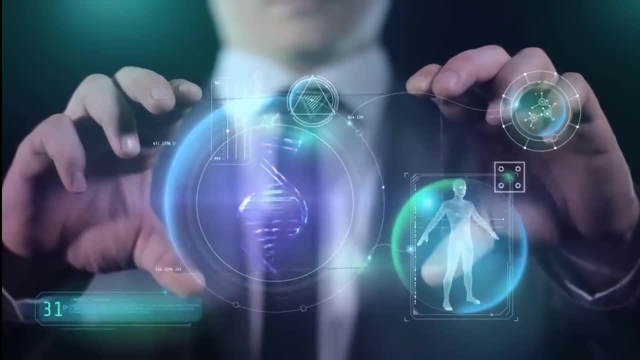 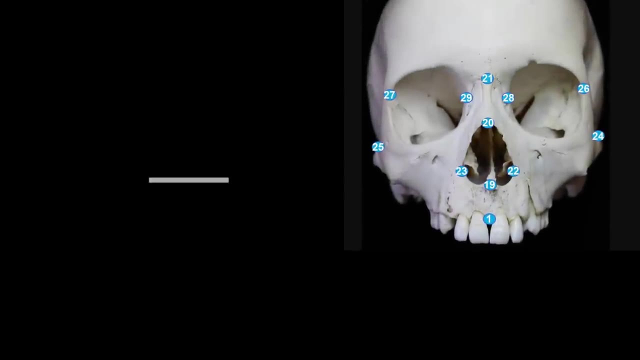 i, a, g, h, a, t term for what have previously been called archaic or primitive Homo sapiens. 500,000 years ago, the other Neanderthals split off from Homo sapiens of that period, where they evolved characteristics that would come to define the Neanderthal lineage. 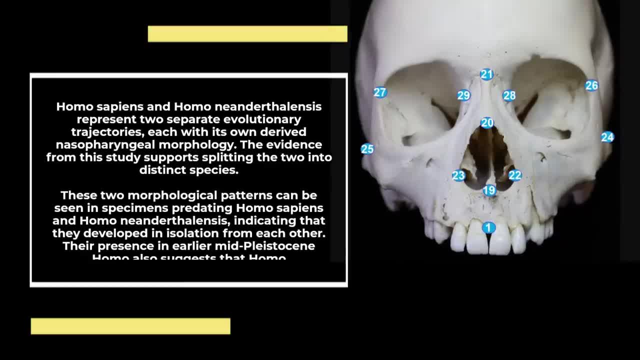 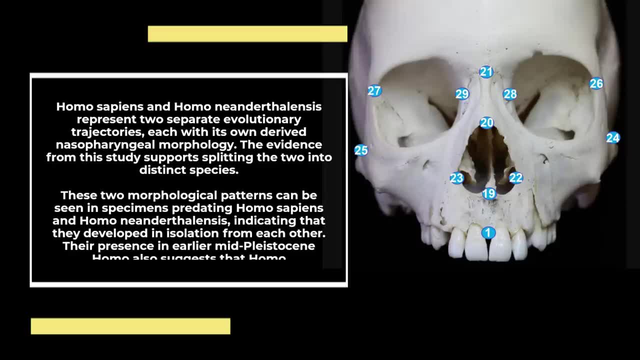 Several hundred thousand years after that, modern humans interbred with the Neanderthals, but even then showed signs of reproductive incompatibility. Because of this, modern humans eventually replaced Neanderthals. The degree of divergence between Neanderthals 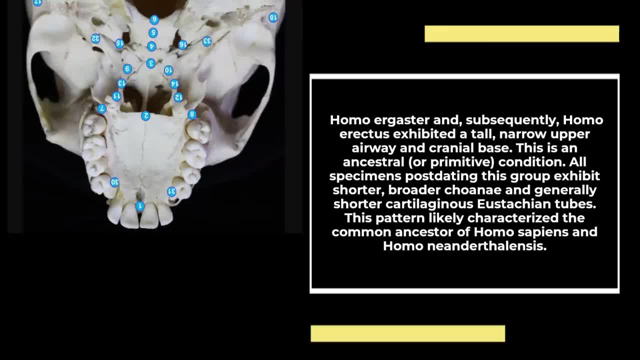 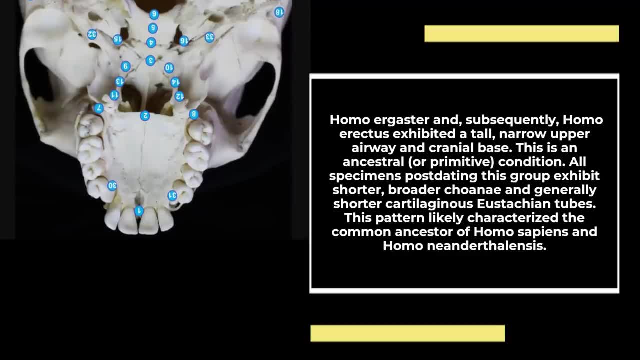 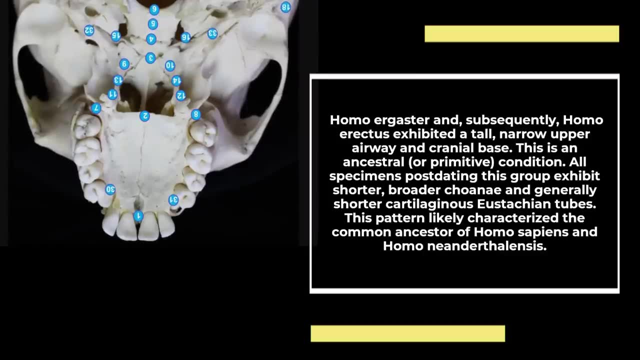 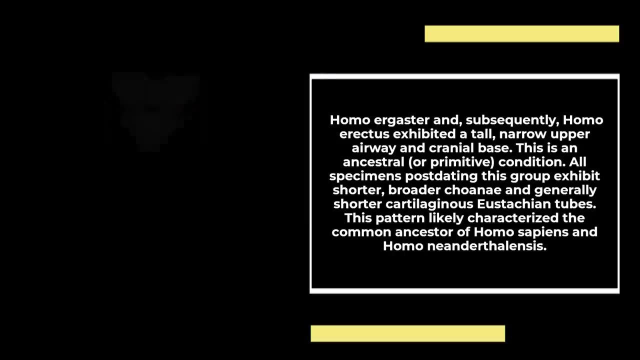 and modern humans over such a short period of time surprised scientists. Why did Neanderthals differentiate so quickly from other early hominins? What pattern of changes did Neanderthals undergo in the process of Neanderthalization? To answer these questions, scientists have needed an accurate picture of European populations. 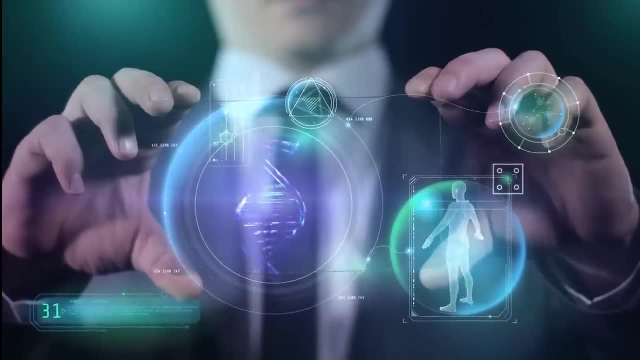 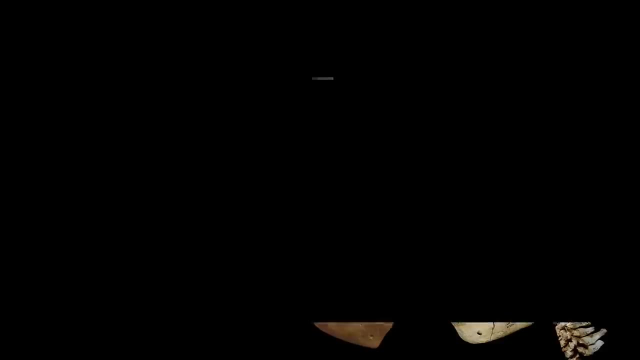 around this time, during the early stages of the Neanderthal lineage and the process of Neanderthalization. This has been challenging because the European fossil record, an important tool for answering these questions, is isolated and dispersed, consisting of remains from 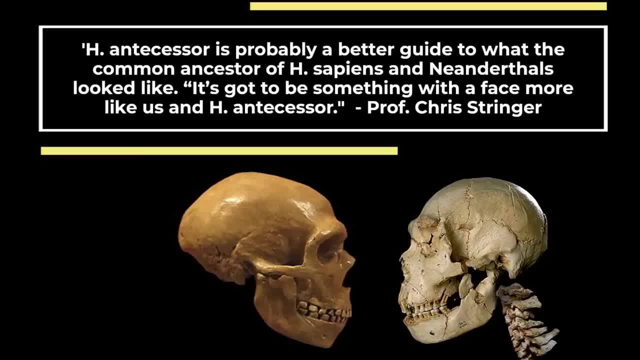 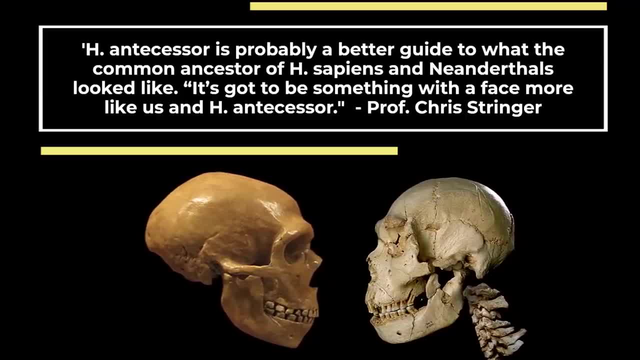 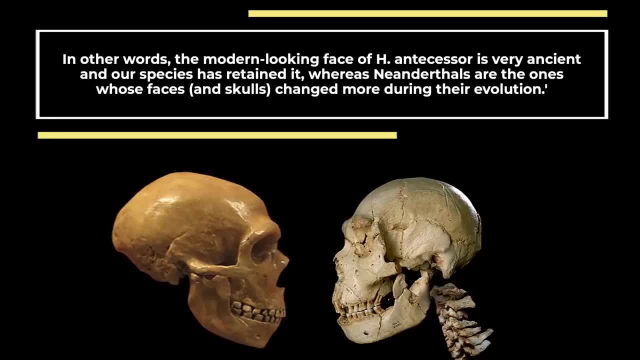 disparate timelines, But samples at the Saima de los Juzos site in Atapuerca, Spain, are different. What makes this site unique is the extraordinary and unprecedented accumulation of hominin fossils there. Nothing quite so large has ever been discovered for any extinct hominin species. 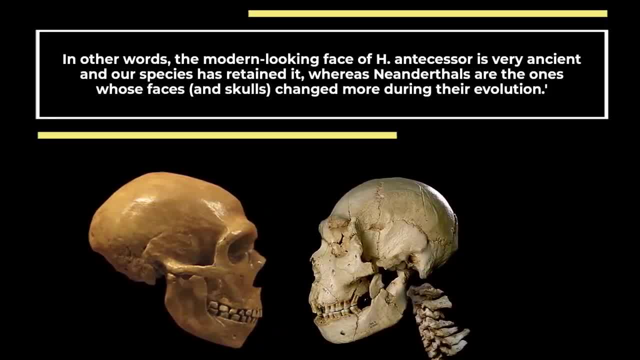 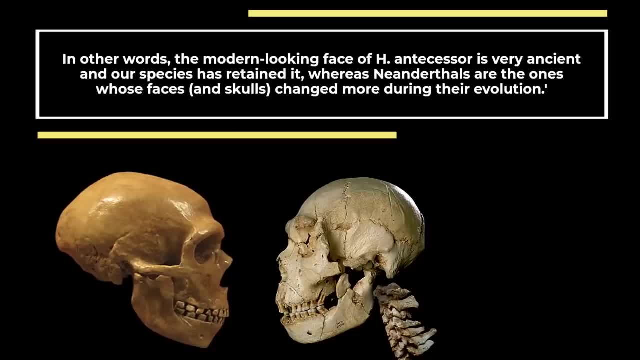 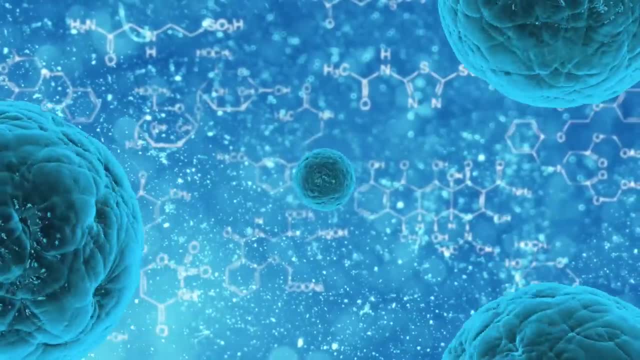 including Neanderthals. This site has been excavated continuously since 1984.. After 30 years, archaeologists have recovered nearly 7,000 human fossils corresponding to skeletal regions of at least 28 individuals. The site's extraordinary collection includes 17 fragmentary skulls, many of which are very complete. 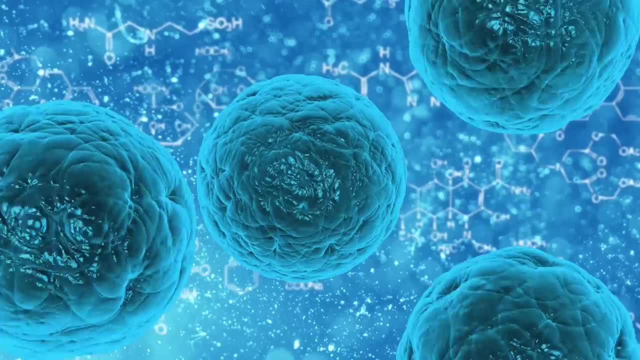 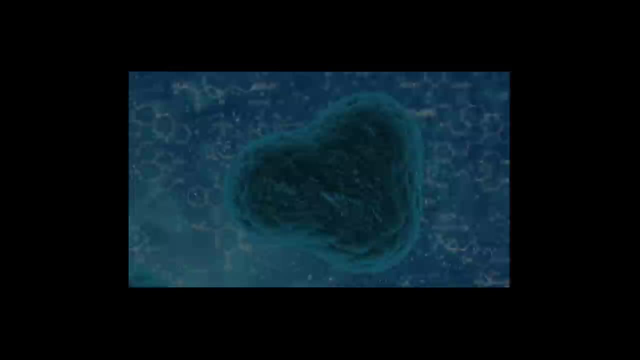 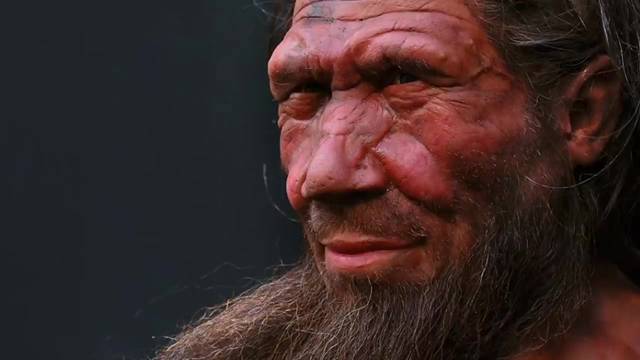 These skulls belong to a single population of a fossil hominin species. Some of them have been studied before, but seven are presented anew and six are more complete than ever before. With these intact samples at their fingertips, anthropologists made progress characterizing their defining features. The work has helped address hypotheses about Neanderthal evolution. 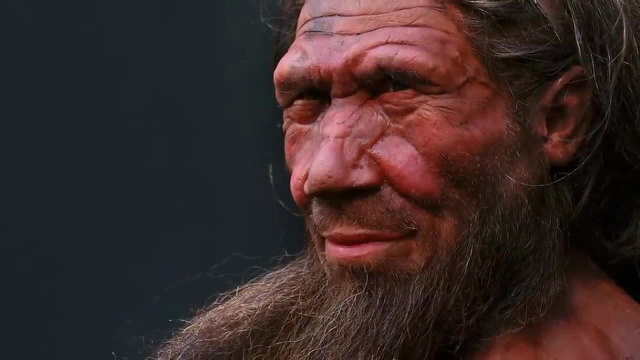 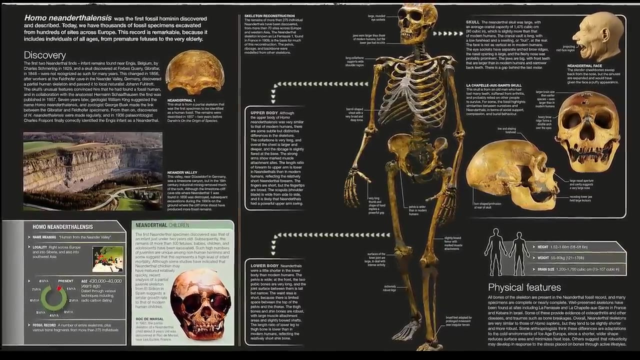 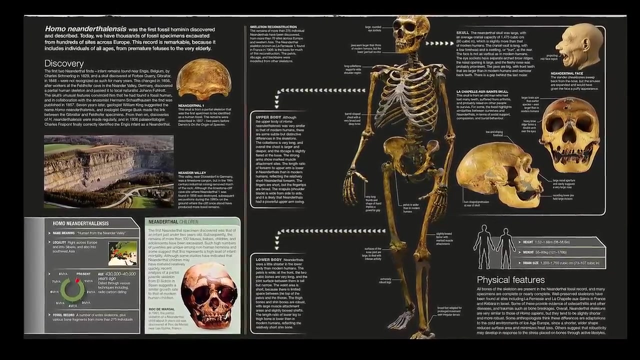 specifically the accretion model hypothesis, which suggests that Neanderthals evolved their defining features at different times, not in a single linear sweep. For decades. the nature of the evolutionary process that gave rise to Neanderthals has been discussed. An important question in these debates was whether the Neanderthalization process involved all regions. 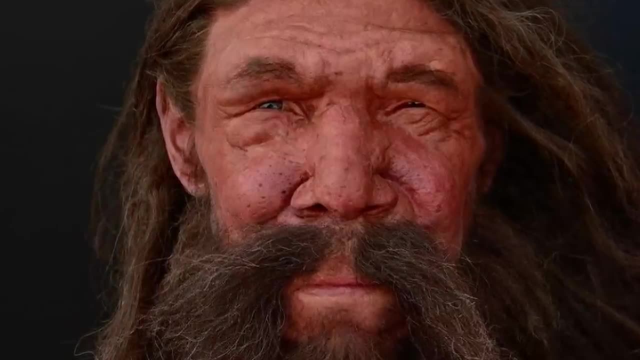 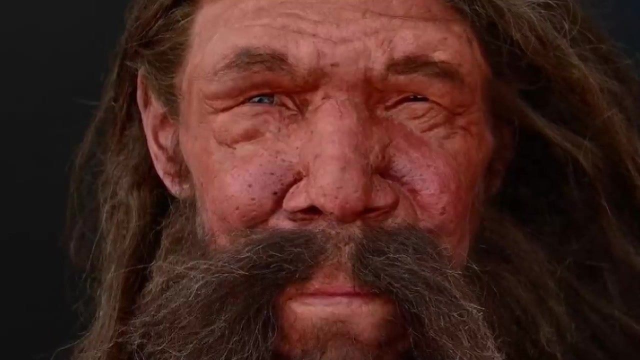 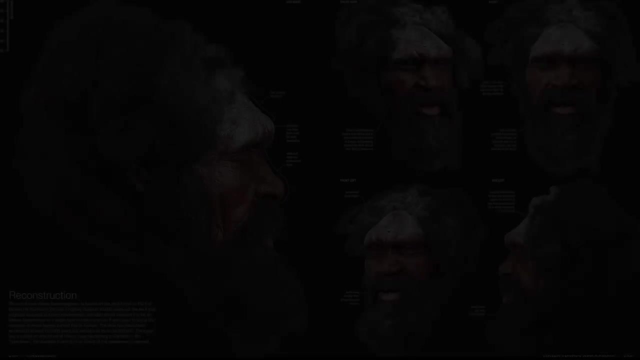 of the skull from the beginning or if there were various stages in this process that affected different parts of the skull at different times. These skull samples showed Neanderthal features present in the face and teeth, but not elsewhere. The nearby brain case, for example, still showed. 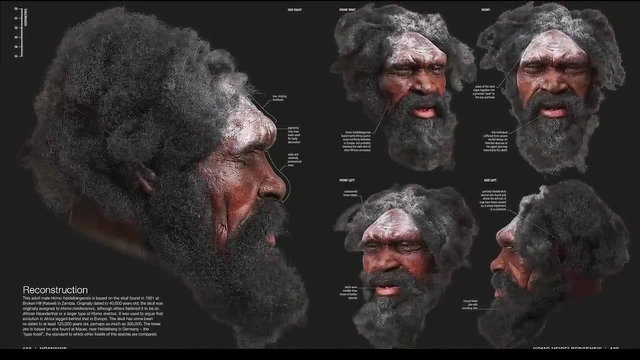 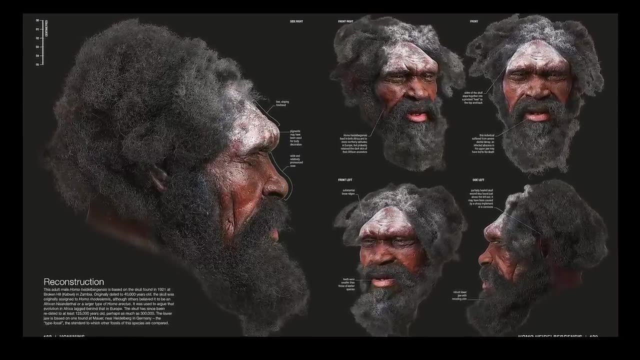 features associated with more primitive hominins. Based on the morphology, researchers concluded that these skulls were part of the Neanderthal clade, although not necessarily direct ancestors to the classic Neanderthals. The Proto-Neanderthal of Spain is a Neanderthal of the Neanderthal clade. The Proto-Neanderthal of Spain is a Neanderthal. 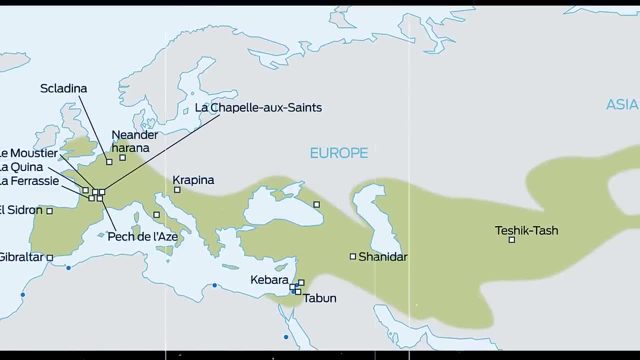 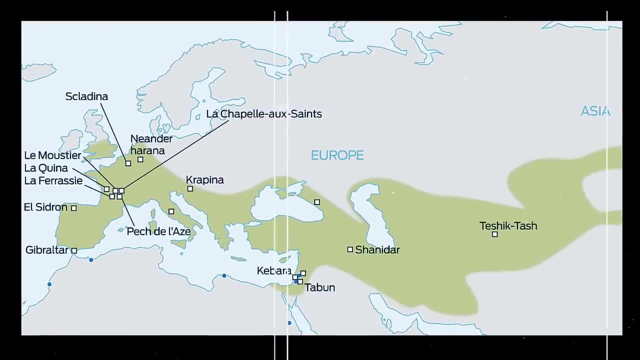 part of an early European lineage that includes Neanderthals but is more primitive than the later Pleistocene variety. Critically, many of the Neanderthal derived features the researchers observed were related to mastication. It seems these modifications had to do with an intensive 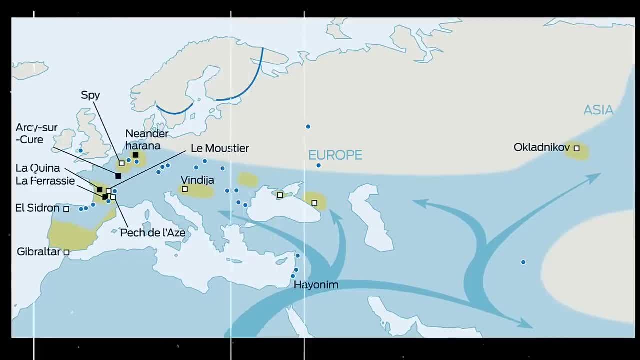 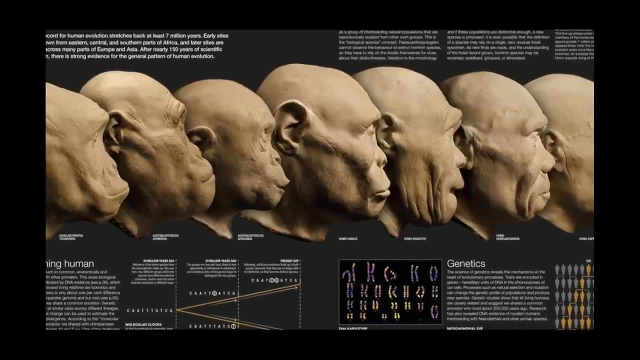 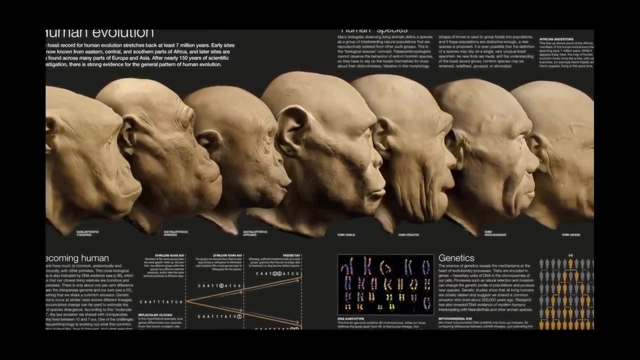 use of the frontal teeth. The incisors show great wear as if they had been used as a third hand, typical of Neanderthals. The study suggests that facial modification was the first step in Neanderthals evolution. Indeed, this mosaic pattern fits the prediction of the accretion model. 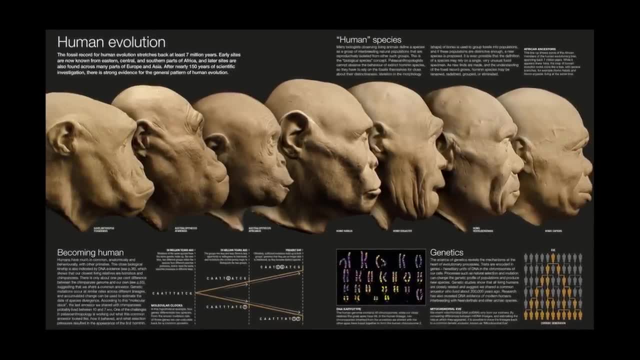 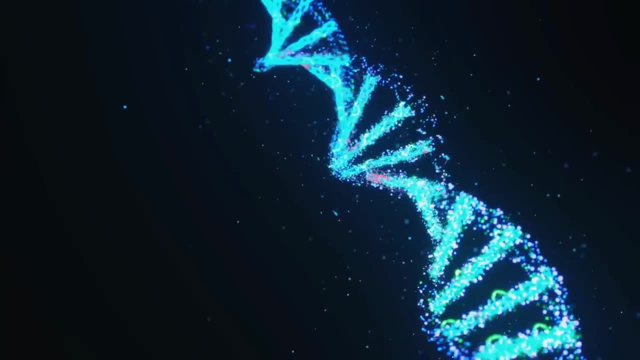 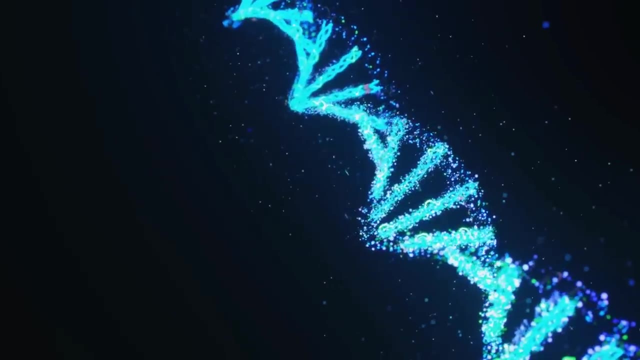 One thing that is surprising about the skulls is how similar the different individuals were. The other fossils of the same geological period are different and don't fit in the Spanish pattern. This means that there was a lot of diversity among different populations in the Middle Pleistocene. In fact, European Middle Pleistocene Homo sapiens do not. 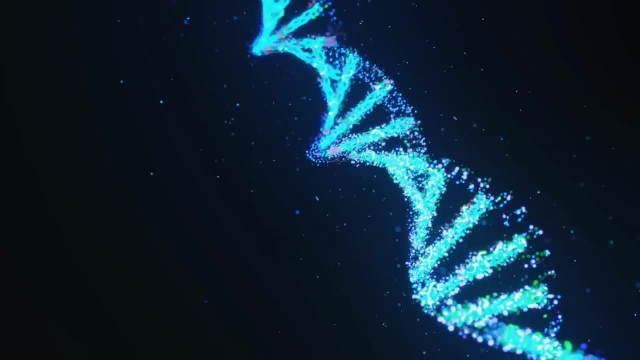 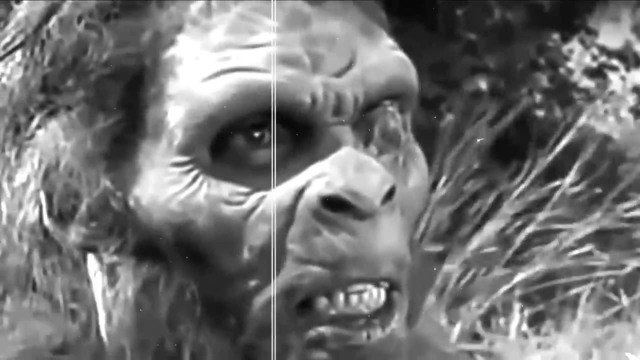 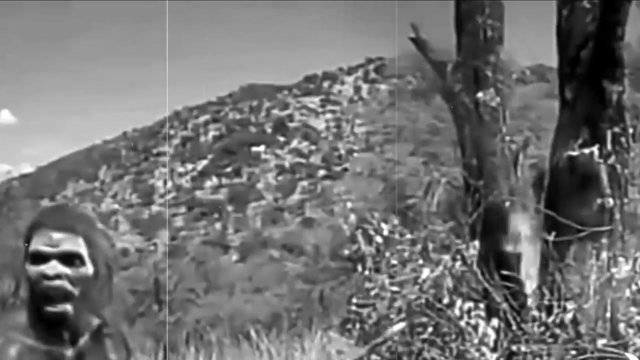 exhibit the suite of Neanderthal-derived features seen in this fossil group. Therefore, more than one evolutionary lineage appears to have coexisted during the European Middle Stone Age, with the Spanish proto-Neanderthals being more closely related to Denisovans than Homo neanderthalensis. Further phylogenetic analysis also backs up the 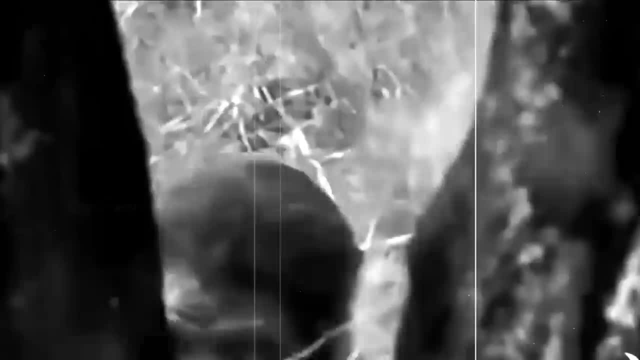 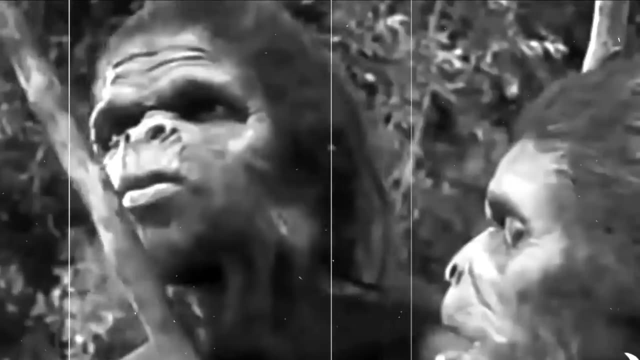 claim that there were two distinct lineages of Neanderthals. This shows that the Spanish proto-Neanderthals and the later classic Neanderthals actually diverged 300,000 years apart. The Spanish proto-Neanderthals split from the line that would give rise to Homo sapiens sapiens. and Neanderthals around 800,000 years ago, while Neanderthals and Homo sapiens split 500,000 years ago. These dates differs from the other study discussed in the first part of the video due to different interpretations of the genetics. 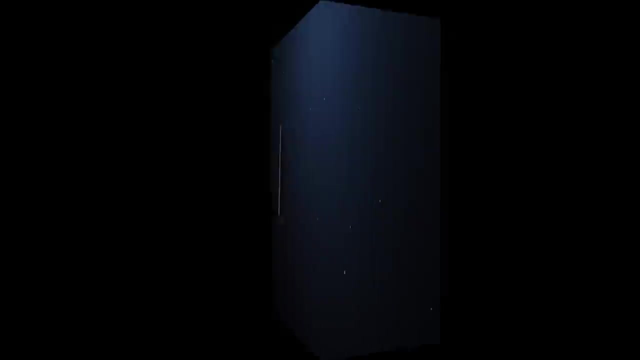 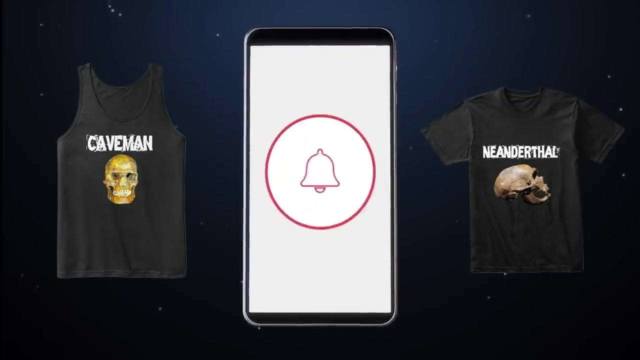 The ancient Neanderthals were not only a shared species of birds, but also known as other birds. We are going to be giving away a t-shirt to a random subscriber this month, so if you find this video compelling, please subscribe, share the video, hit the like button and leave a comment or suggestion. 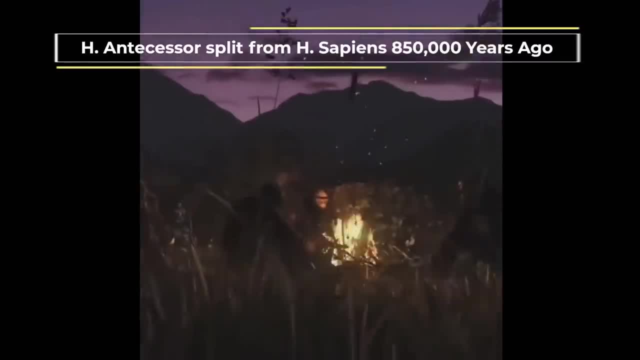 However, another piece of the puzzle is Homo antecessor, who lived in Spain more than 400,000 years prior to the proto-Neanderthals. When discovered, Homo antecessor is the first species to have a sputum in the Neanderthal family, The sputum which is the. most common is the first of the three species to have a sputum in the Neanderthal family. The sputum is the second of the three species to have a sputum in the Neanderthal family. The sputum was the first to have a sputum in. 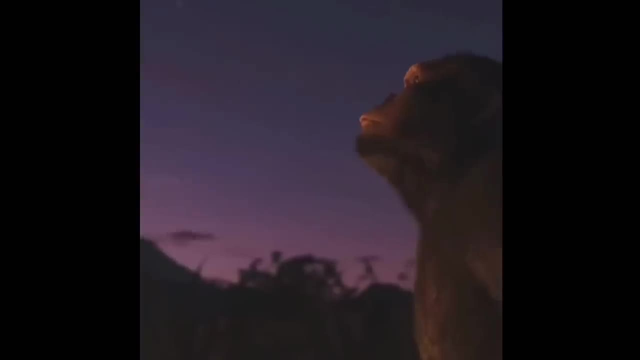 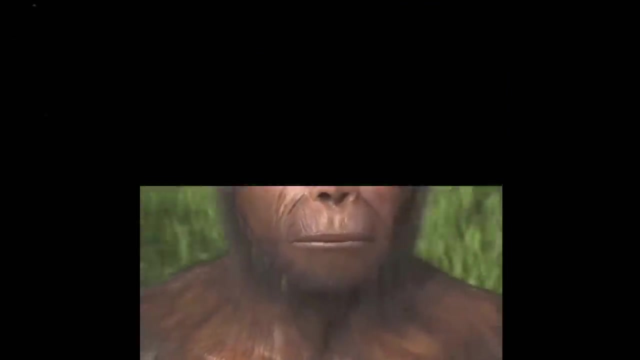 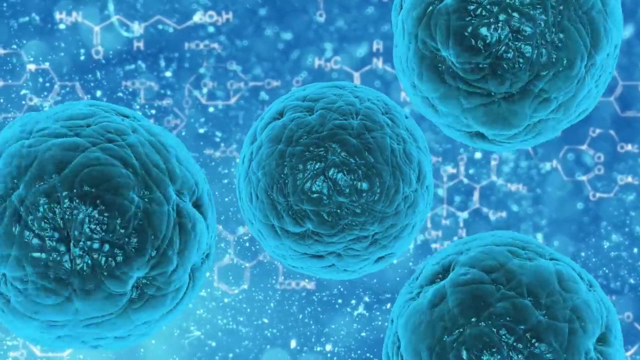 was tentatively proposed as the last common ancestor of Neanderthals and modern humans. In fact, lurking deep in your DNA, you may have a ghostly remnant from this super-archaic proto-human that isn't our ancestor. This is because, over half a million years ago, 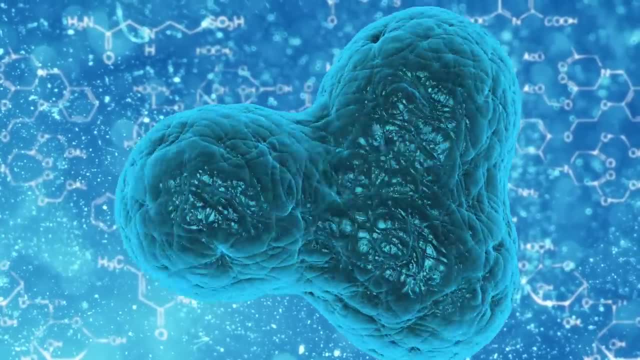 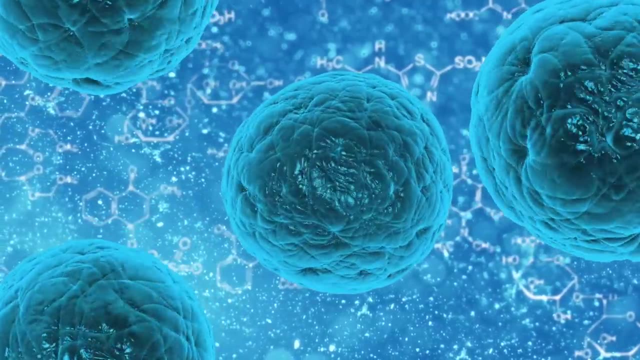 Neanderthals, the common ancestor of proto-Neanderthals and Denisovans, may have intermixed with Homo Anticessa and then in turn mated with archaic Homo Sapiens. Scientists demonstrated that Homo Anticessa is a close sister lineage to hominins such as: 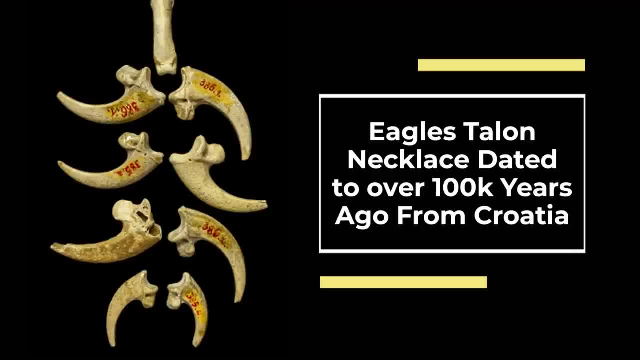 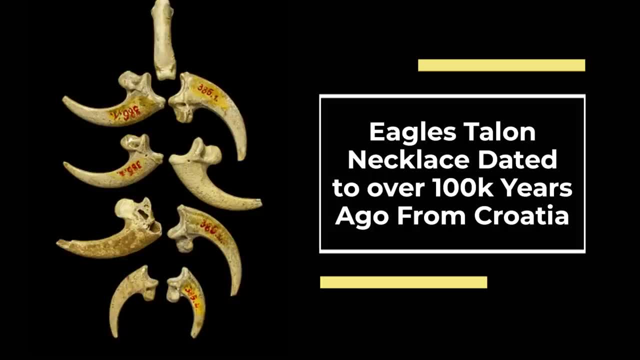 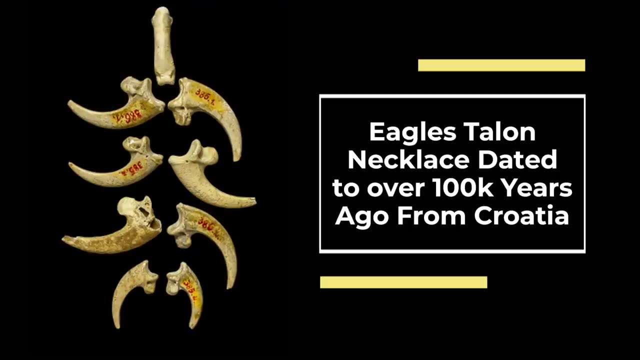 modern humans, Neanderthals and Denisovans. This placement implies that the modern-like face of Homo Anticessa may have a considerably deep ancestry in the genus and that the Neanderthal cranial morphology represents a derived form. The relationships of this species to earlier. 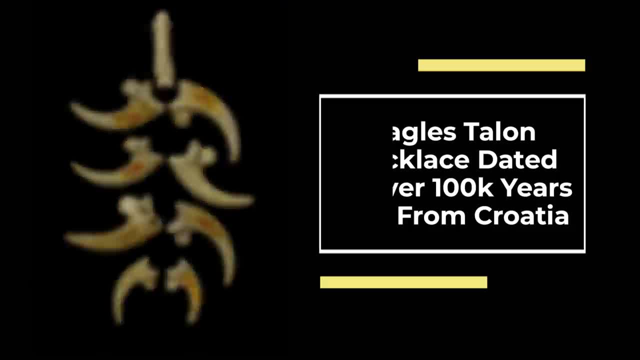 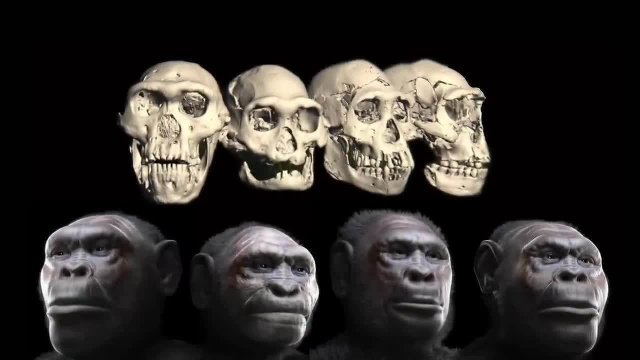 hominins in Eurasia, such as the Homo erectus specimens from Dmanisai, Georgia, and to later hominins in Eurasia are very similar. These issues had remained unresolved due to the fragmentary nature of hominin fossils at other 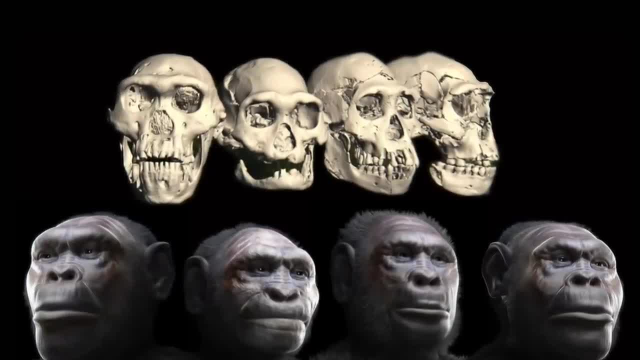 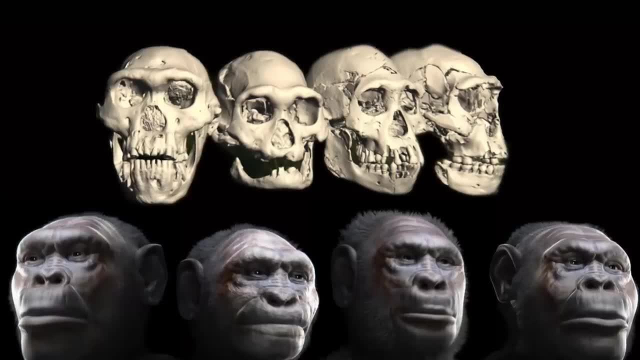 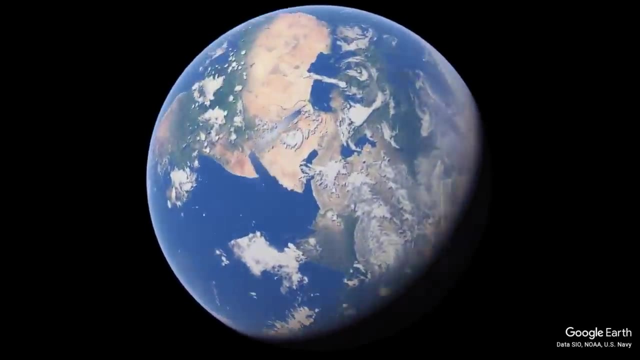 sites and the failure to recover ancient DNA in Eurasia. Homo Anticessa is only known from the Grand Olena assemblage in Atapuerca, Spain. Its relationship with other European Middle Pleistocene fossils is heavily debated. It is still contentious whether Homo Anticessa could represent the last common ancestor of 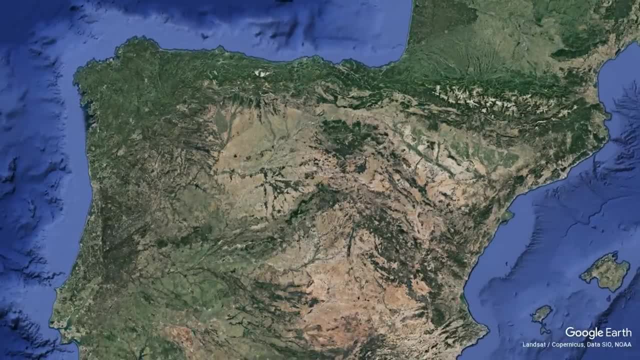 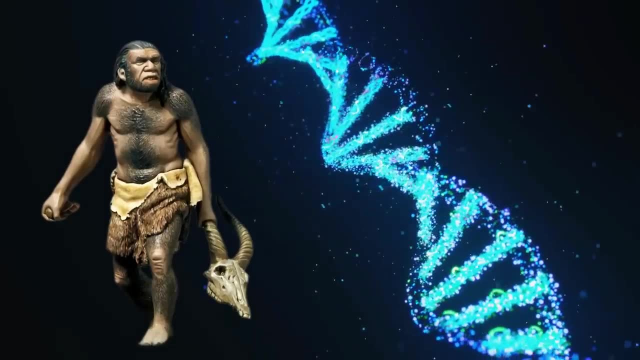 Homo Sapiens, Neanderthals, Neanderthals and Denisovans, or whether it represents a sister lineage to the last common ancestor of these species. Fossils from northern Algeria, in Africa, dated to 700,000 years ago and known as Homo. 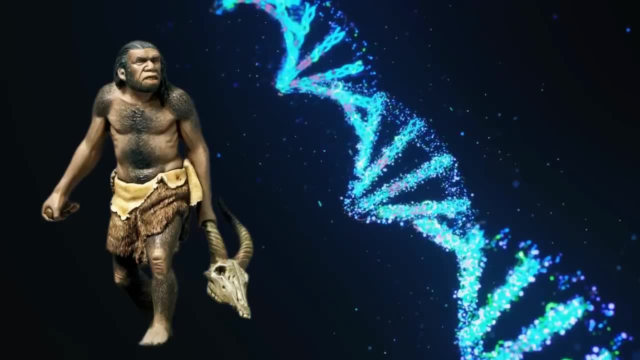 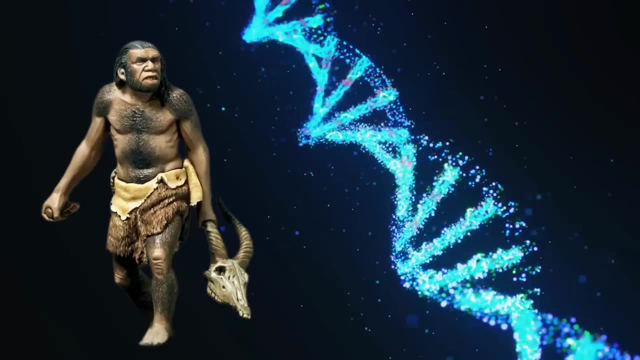 mauritanicus have also been suggested to be Homo Anticessa, based on dental similarities. But how did Homo Anticessa cross the Mediterranean? Did they use boats? Anything is possible at this point. Another study suggests that Homo Anticessa is a species of Homo sapiens.